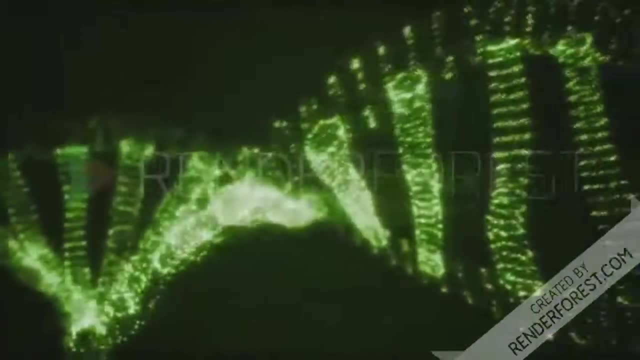 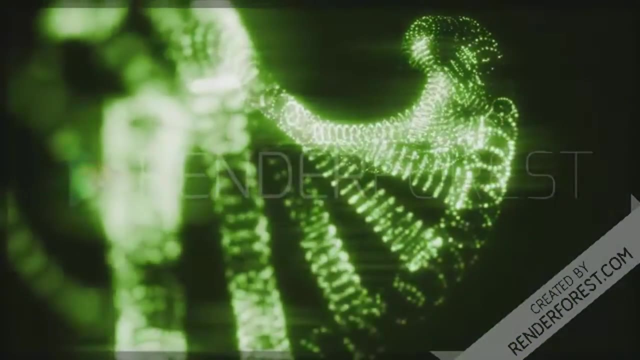 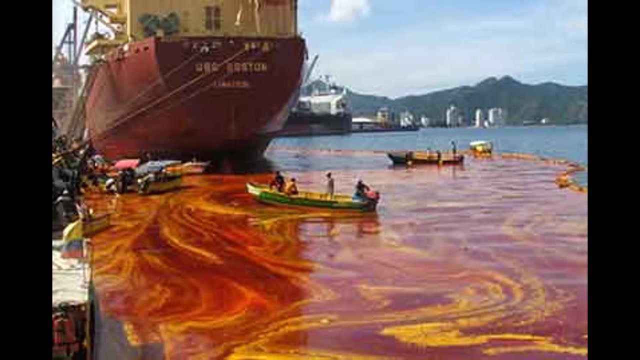 Most water pollutants are eventually carried by rivers into the oceans. In some areas of the world, the influence can be traced hundred miles from the mouth by studies using hydrology transport models. Advanced computer models such as SWMM or the DSOM model have been used. 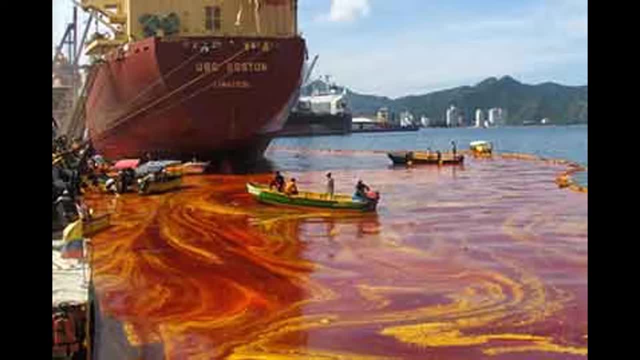 in many locations worldwide to examine the fate of pollutants in aquatic systems. Indicator filter feeding species such as cope ponds have also been used to study pollutant fates. in the New York Bight, for example, The highest toxin loads are not directly at the mouth. of the Hudson River, but 100 km south, since several days are required for incorporation into planktonic tissue. The Hudson discharge flows south along the coast due to coriolis force. Further south, then are areas of oxygen depletion caused by chemicals using up oxygen. 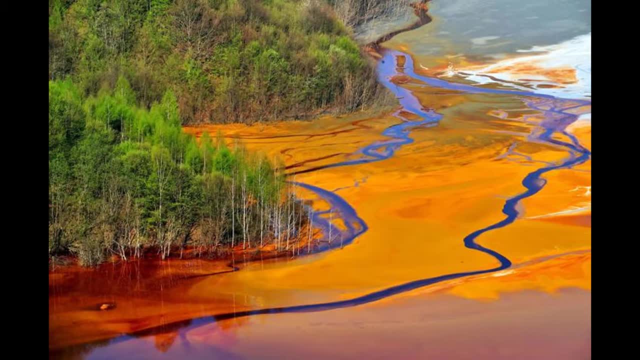 and by algae blooms caused by excess nutrients from algal cell death and decomposition. Fish and shellfish kills have been reported because toxins climb the food chain: after small fish consume cope pods, then large fish eat smaller fish, etc. Each successive step up the food. 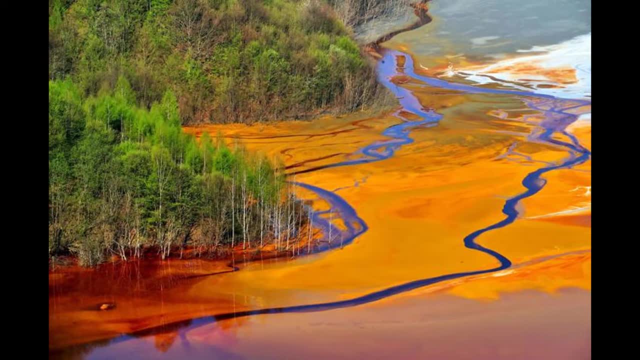 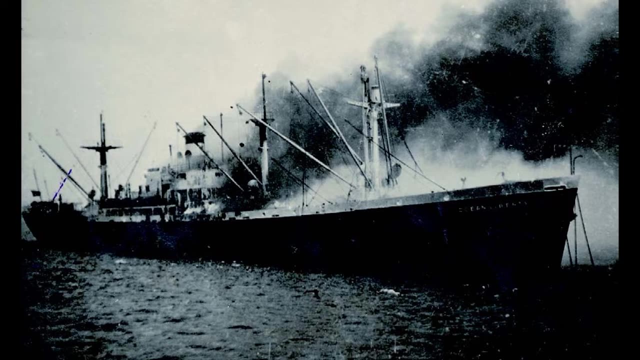 chain causes a stepwise concentration of pollutants such as heavy metals, for example mercury, and persistent organic pollutants such as DDT. This is known as biomagnification, which is occasionally used interchangeably with bioaccumulation. Example: a polluted river draining an abandoned copper mine on Anglesey- large gyres, vortexes. 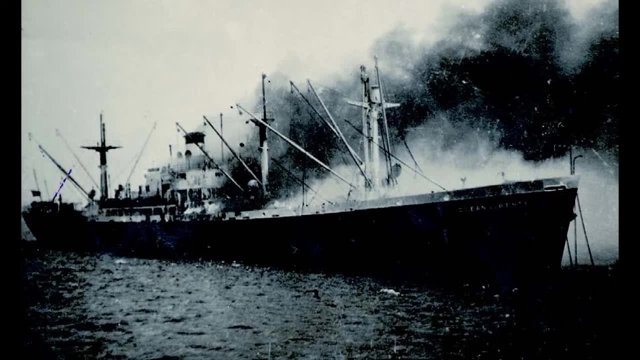 in the ocean's trap floating plastic debris. The North Pacific Gyre, for example, has collected the so-called Great Pacific Garbage Patch that is now estimated at 100 times the size of Texas. Many of these long-lasting pieces wind up in the stomachs of marine birds and animals. This results 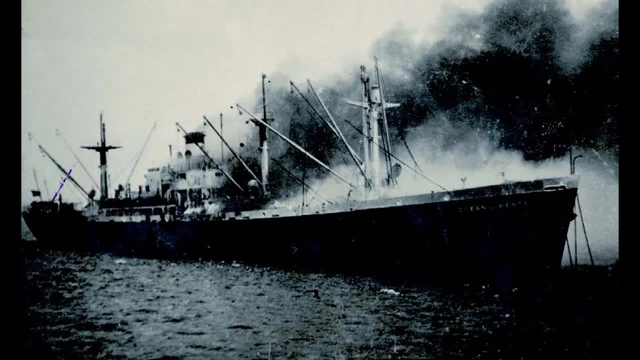 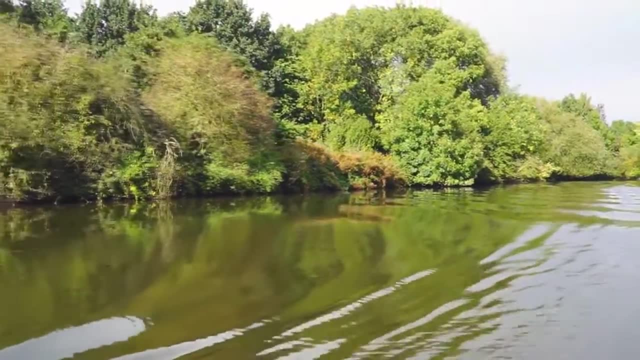 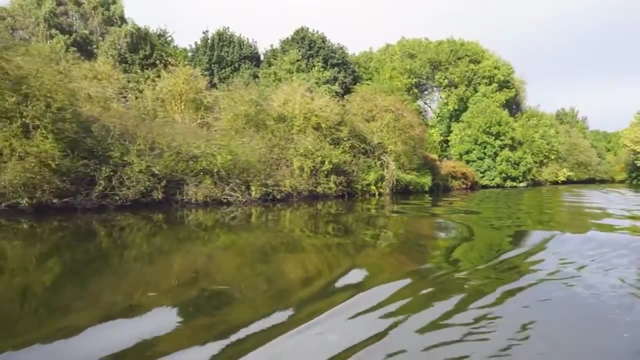 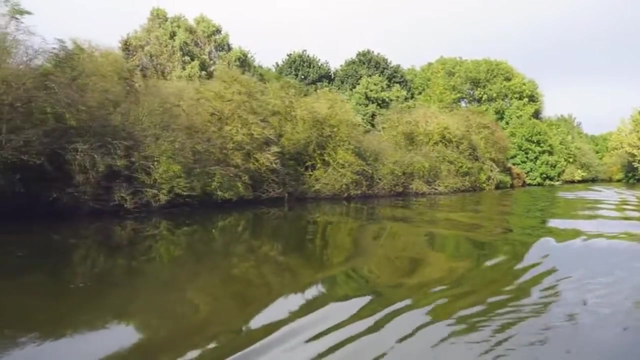 in obstruction of digestive pathways, which leads to reduced appetite or even starvation. Many chemicals undergo reactive decay or chemically change, especially over long periods of time in groundwater reservoirs. A noteworthy class of such chemicals is the chlorinated hydrocarbons, such as chloroethylene, used in industrial metal degreasing and electronics manufacturing, and tetrachloroethylene.